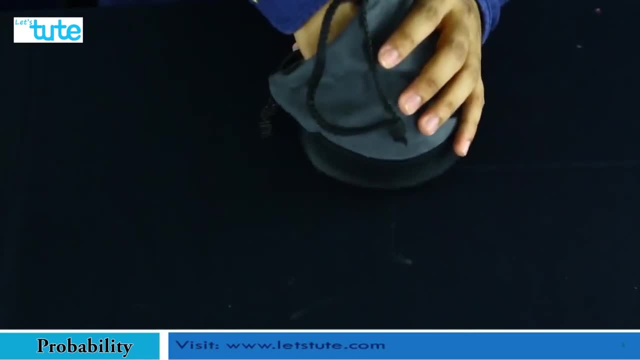 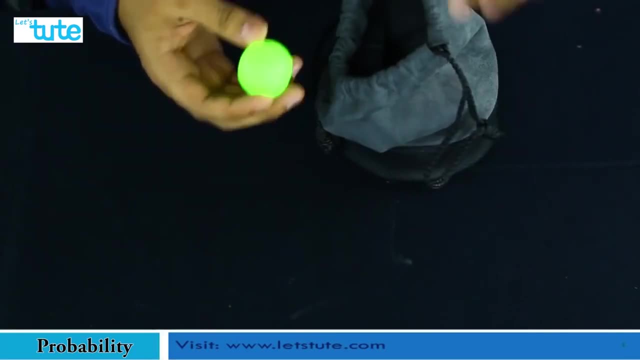 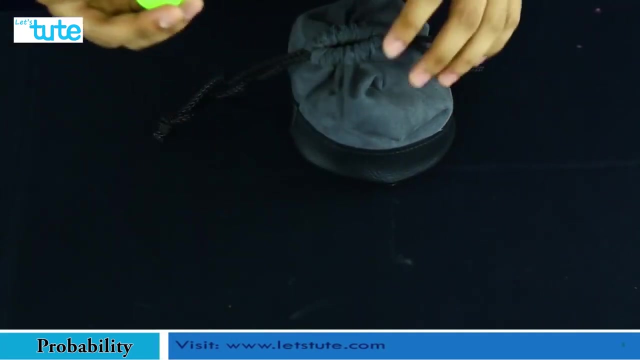 one ball. okay, and I do not know which ball it is going to be, because I cannot really see the color. Suppose I take out a ball and I get a fluorescent ball. So now I want to check the probability of getting this fluorescent ball. Like, how many times will I get this fluorescent? 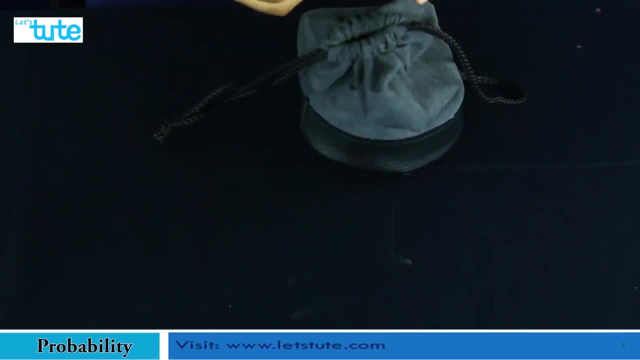 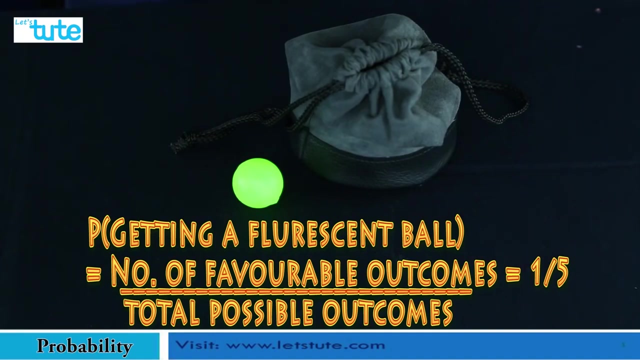 ball whenever I would put a hand inside and I would try to take out a ball. We can calculate that by a formula: Number of outcome favorable to fluorescent ball, number of outcomes favorable to fluorescent ball and number of outcomes favorable to fluorescent ball divided by total number of possible outcomes. So this would give me 1 divided by 5,. 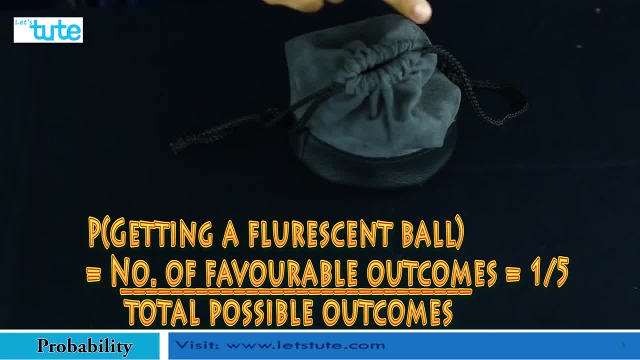 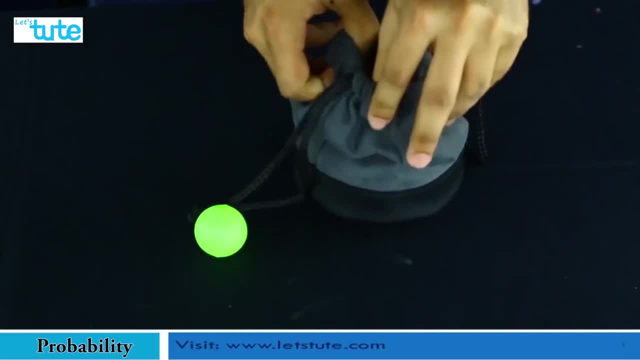 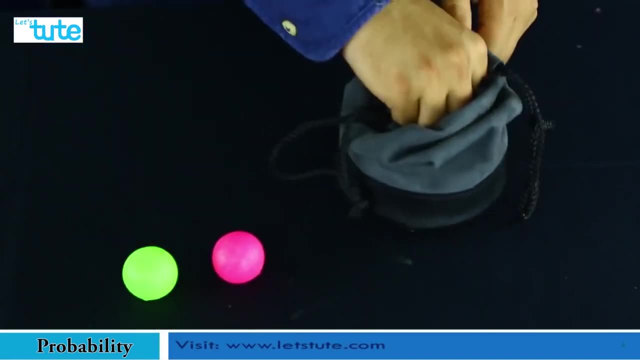 1, because there is only one ball, one fluorescent ball, among these five balls. So the sum of the probabilities rule should satisfy this experiment. So now I said this has 1 by 5 probability. this will have 1 by 5 probability. this will have 1 by 5 probability. 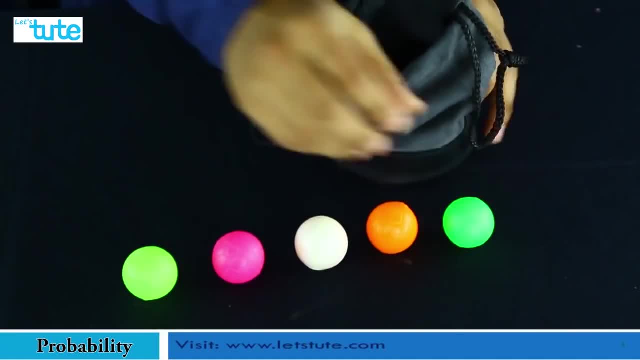 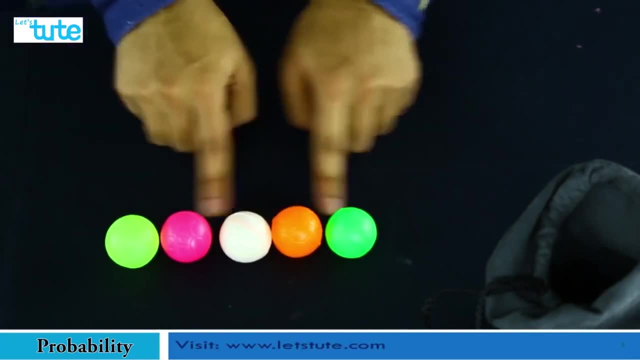 this will have 1 by 5 probability. This has 1 by 5 probability. this will have 1 by 5 probability, this will have 0 probability, and even this will have 1 by 5 probability. So now, if we are going to add all the probabilities, 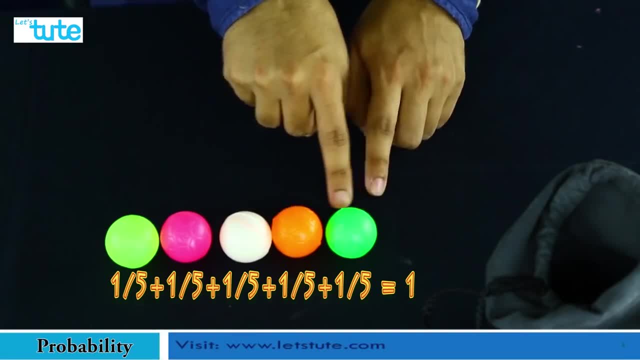 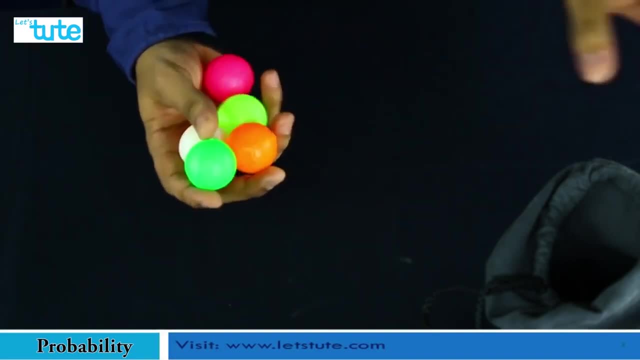 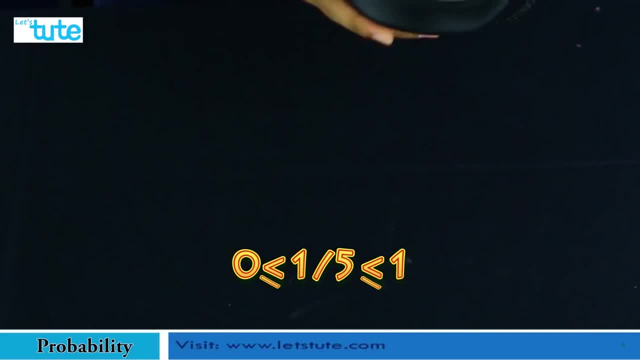 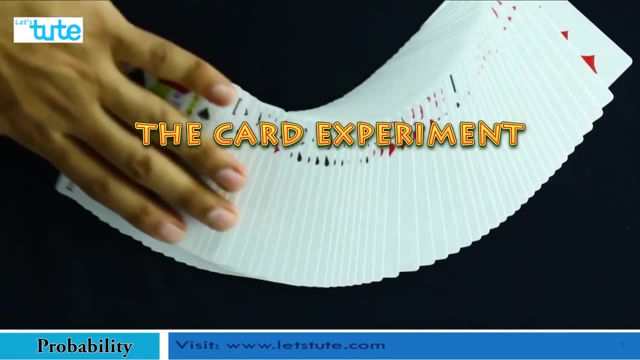 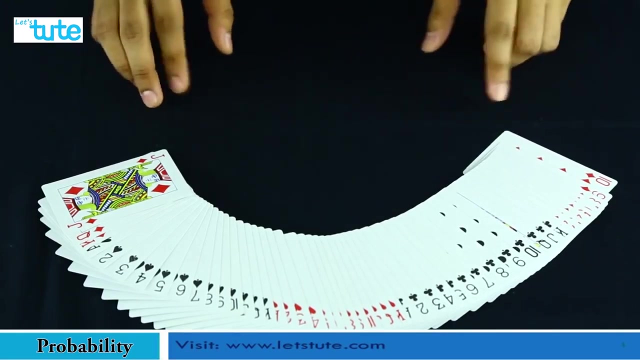 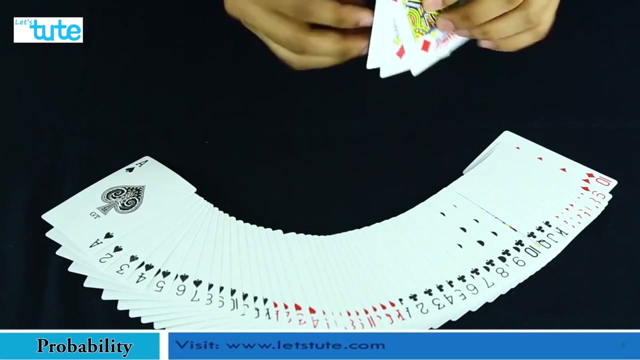 0 and 1.. So it again satisfies all the rules. So the ball experiment is over. In a pack of card we have 52 cards in a deck and that forms one pack or one deck. In that we have three phase cards, namely a king, a queen, a king, a queen, a king, a queen, a 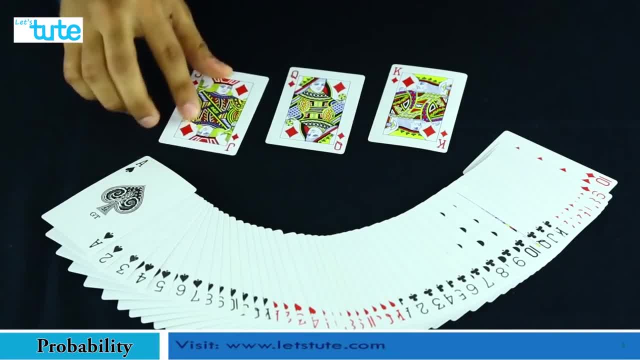 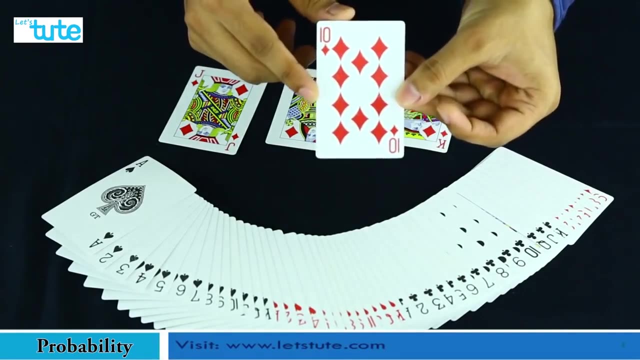 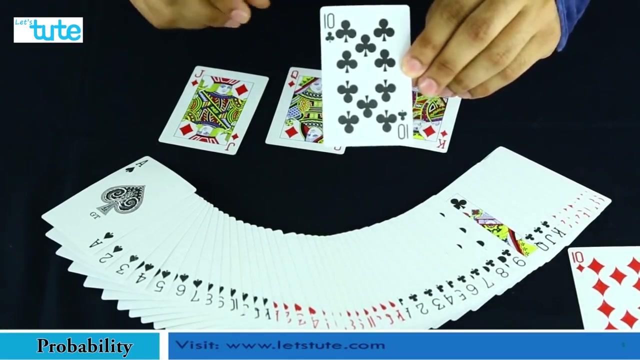 king and a jack. These are the three phase cards that we have And we have four suits and each suit is represented by a shape or a color. We have one suit called diamond, and this is red in color. We have one suit, club, which is black in color. We have one suit called heart, which is green. 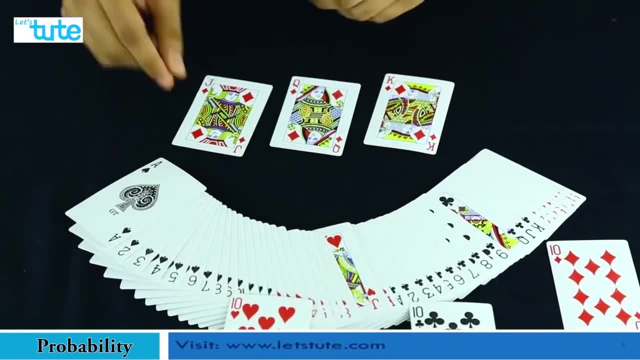 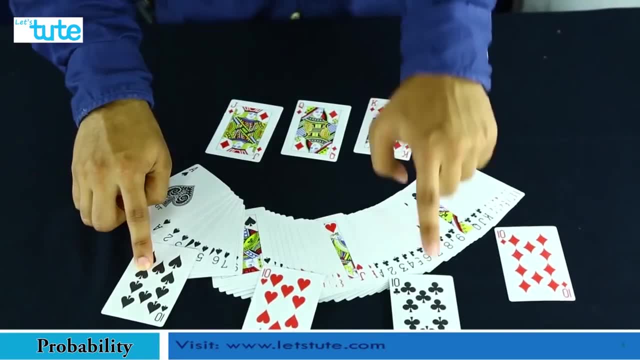 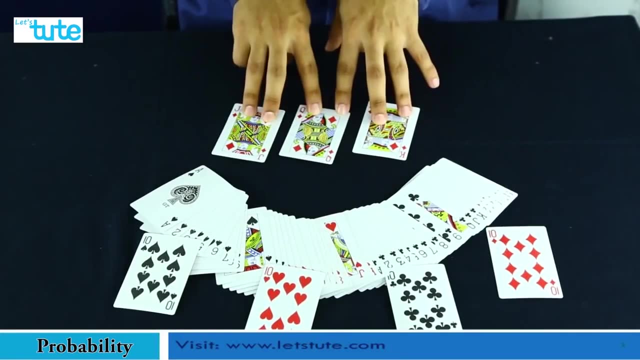 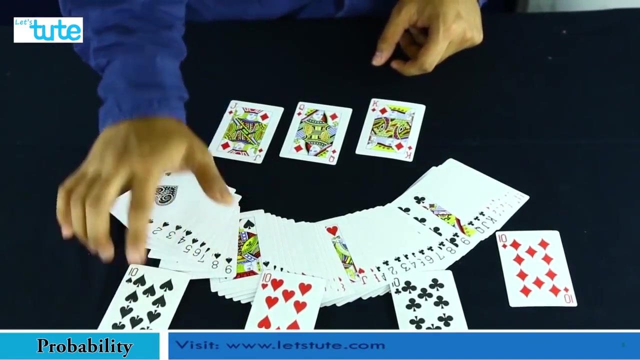 again red in color, and we have one suit- spades- that is black in color. So the spades and the club is black in color and the heart and the diamond is red in color. There are 4 suits with 3 face cards and the other numbers are ace, 2,, 3,, 4,, 5,, 6,, 7,, 8,, 9 and 10. all right, 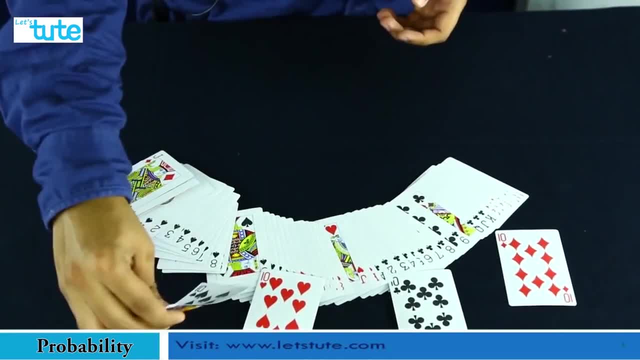 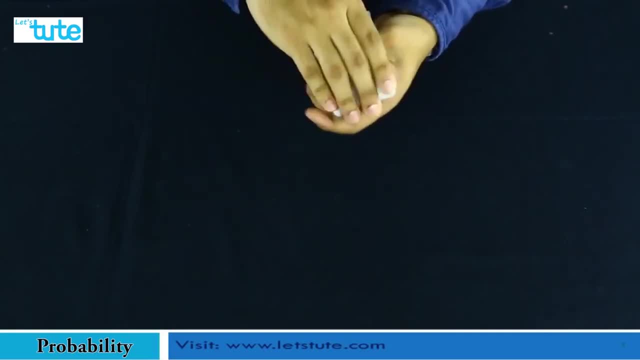 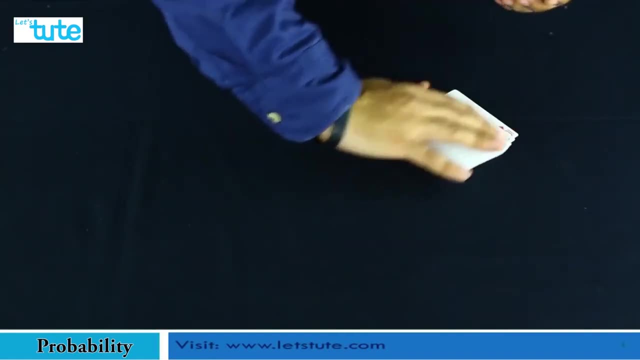 So this is how the number goes. Now suppose we have this deck of cards, well shuffled. ok, I am shuffling these cards because before it was arranged in a color wise manner, So I am shuffling these cards- we had 52 number of outcomes. ok, From these 52 we want to take: 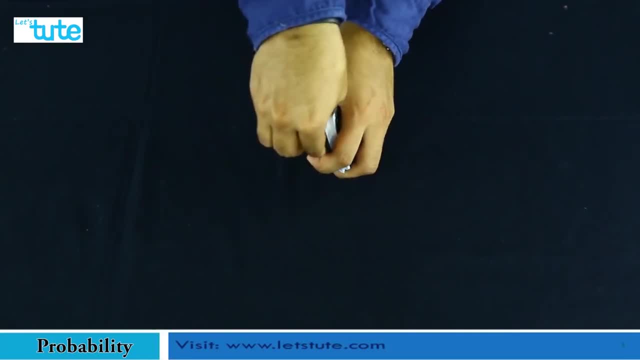 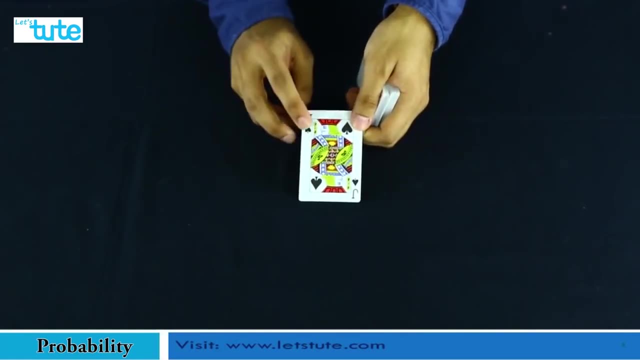 out one card. ok, I am not looking at these cards and I take out any one card. ok, any one. Suppose I have jack of all cards, Jack of spades, ok. So what should I do To calculate the probability of getting a? 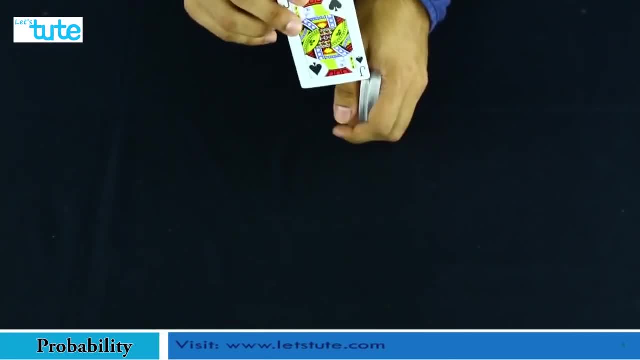 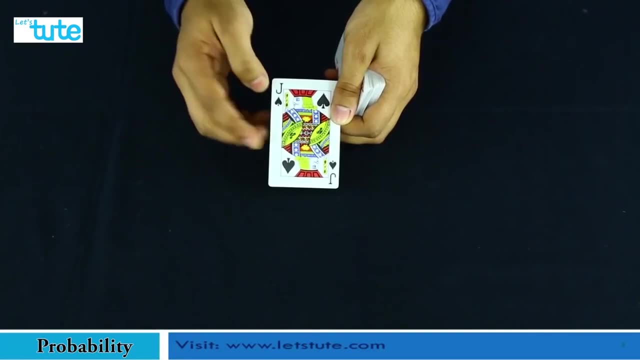 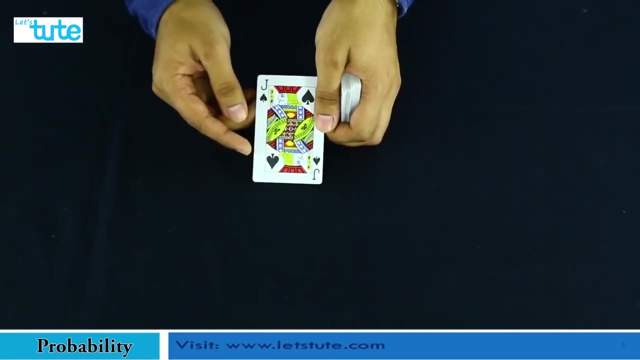 jack of spades from these 52 cards and I cannot say that it is biased, because there is, yes, there is different jack, but then it is of different suit and different color. So this experiment is again not biased and has equally likely outcomes. So to get a black jack from 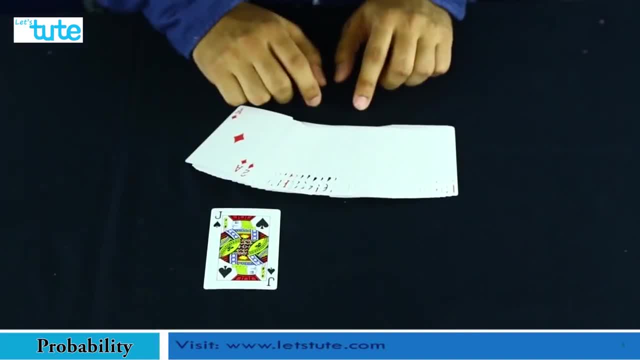 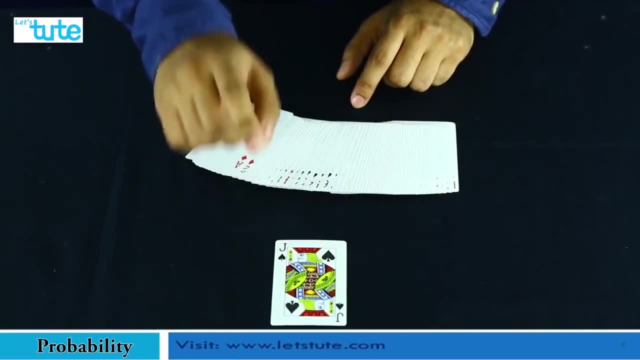 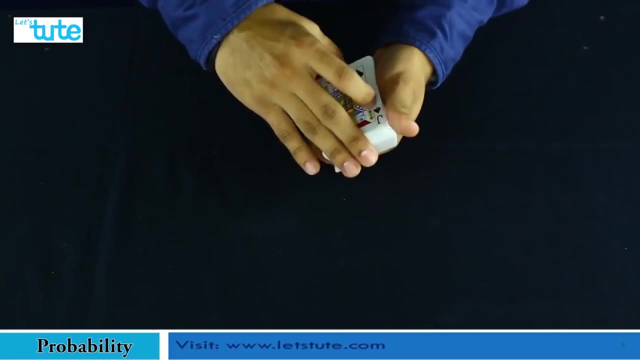 these Set of 52 cards, what is the probability? Number of outcomes favorable to get a black jack or a jack of spades is equal to 1 and total number of outcomes as 52. So it becomes 1 upon 52. Now we have to see if it satisfies the sum of probabilities rule. Each card will 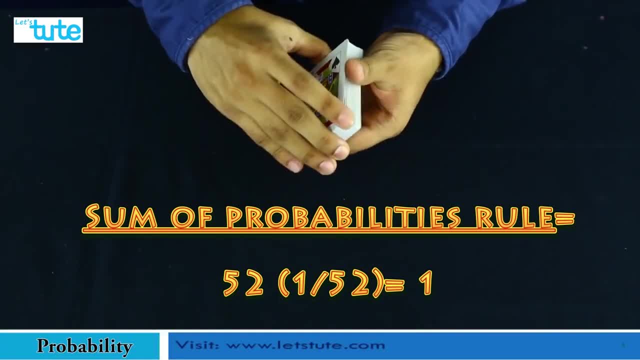 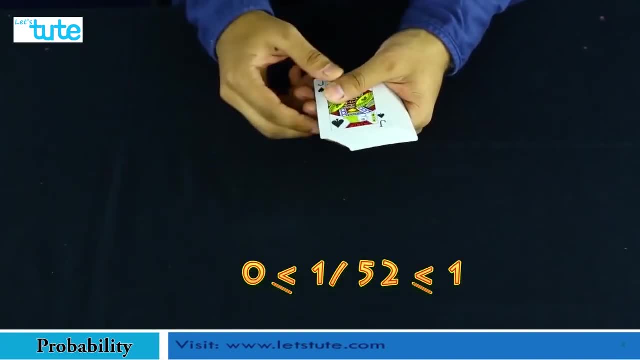 have 1 upon 52. So we will add all these cards and it will make make up to 1, and again, 1 upon 52 is And that means it makes up to 1.. Now we can also take out the rest of the yarns on top. 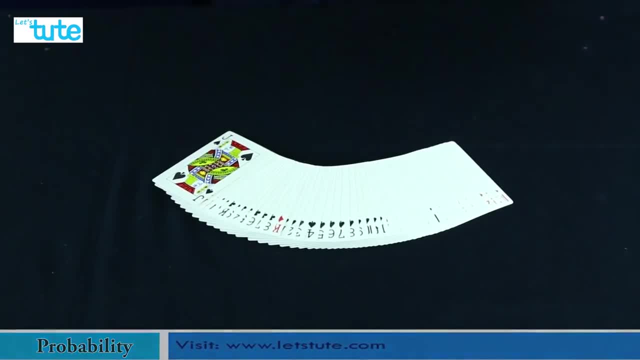 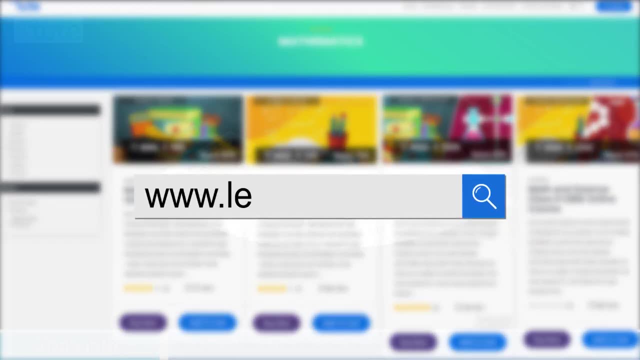 of this curve. So the total number of Verb is equal to 1 and the number of Advanced numbers equal to 1, and that means only the 1-2 is between 0 and 1.. So it is definitely going to satisfy the rule that we already discussed.